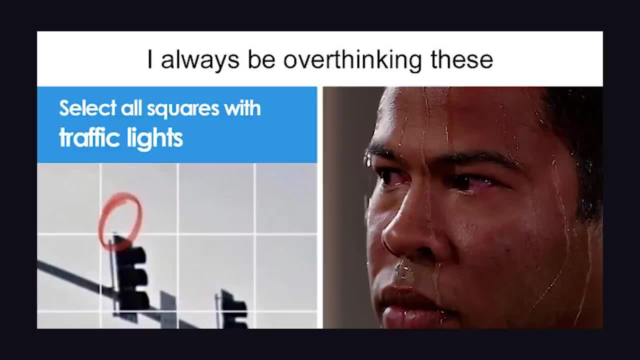 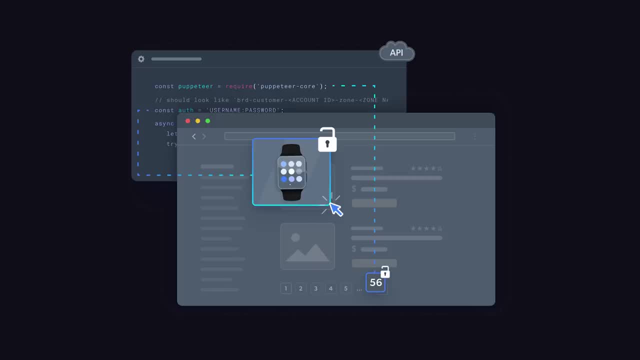 and will block your IP address or make you solve captchas if they suspect you're not a human. But that's kind of racist to non-biological life. Luckily, BrightData, the sponsor of today's video, provides a special tool called the Scraping Browser. It runs on a proxy network and provides 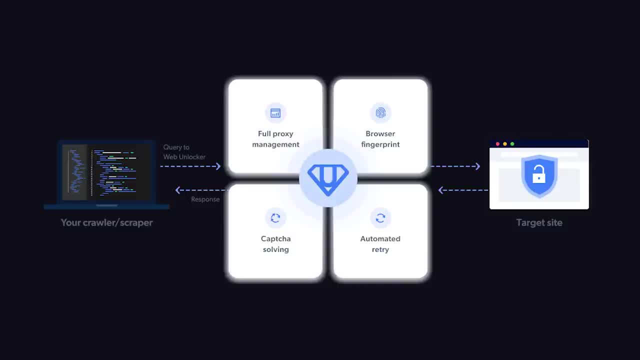 a variety of built-in features, like captcha solving fingerprints, retries and so on, that allow you to scrape the web at an industrial scale. That being said, if you're serious about extracting data from the web, you're going to have to be very careful. If you're not. 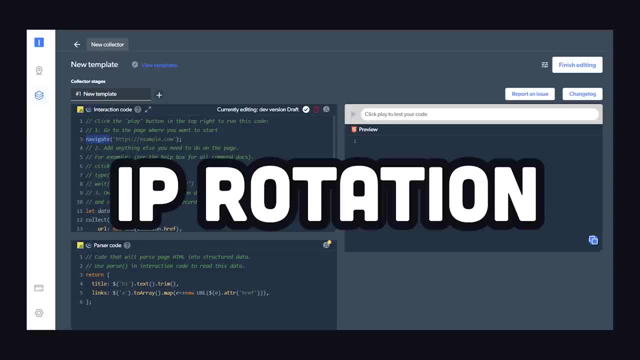 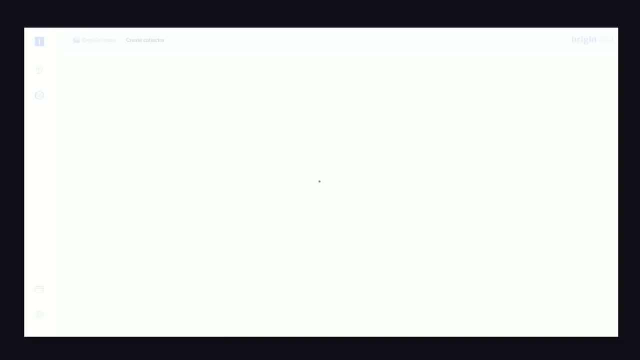 you'll very likely need a tool that does automated IP address rotation, and you can try BrightData for free using this code. After you sign up for an account, you'll notice a product called the WebScraper IDE. We're not going to use it in this video. However, if you're serious, 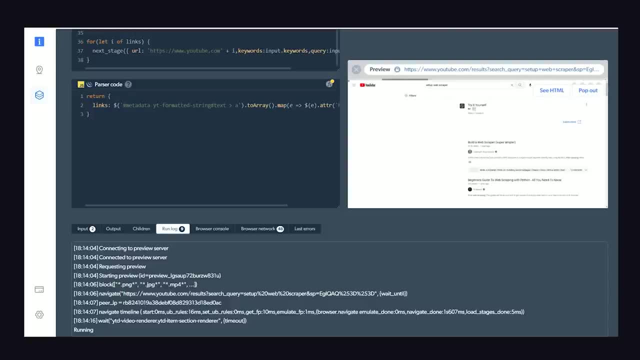 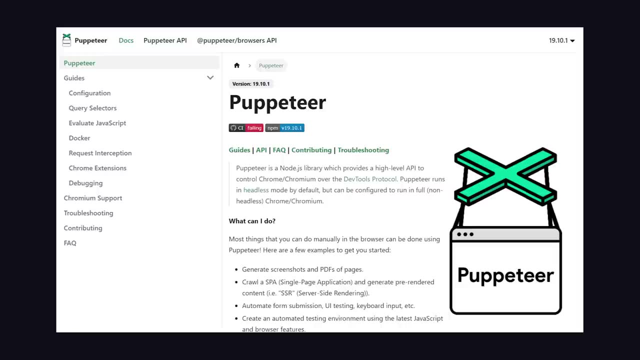 about web scraping. it provides a bunch of templates and additional tools that you'll likely want to take advantage of. As a developer myself, I want full control over my workflow, So for that I'm going to use an open source tool from Google called Puppeteer, which is a 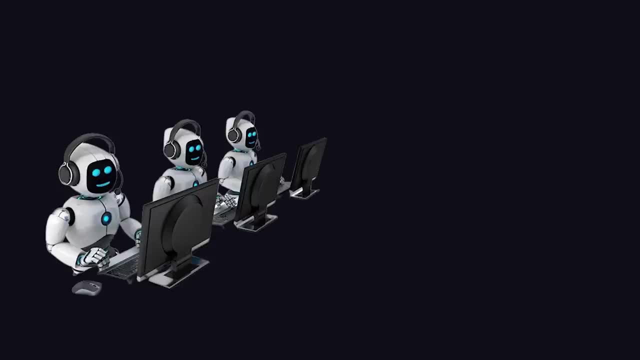 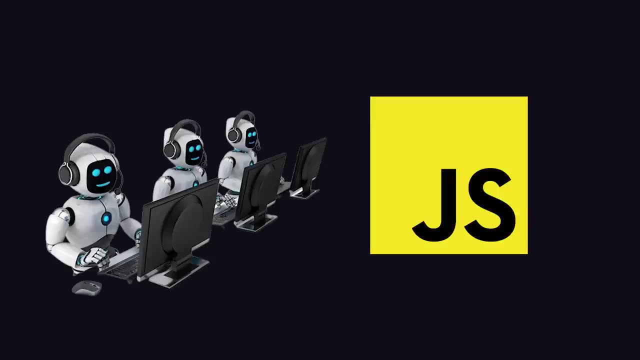 headless browser that allows you to view a website like an end user, to interact with it programmatically using JavaScript, clicking on buttons and doing everything else a user can do. That's pretty cool, but if you use it a lot on the same website, they'll eventually flag your IP and ban you from. 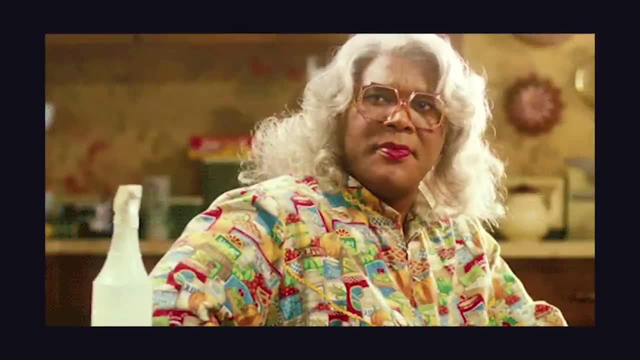 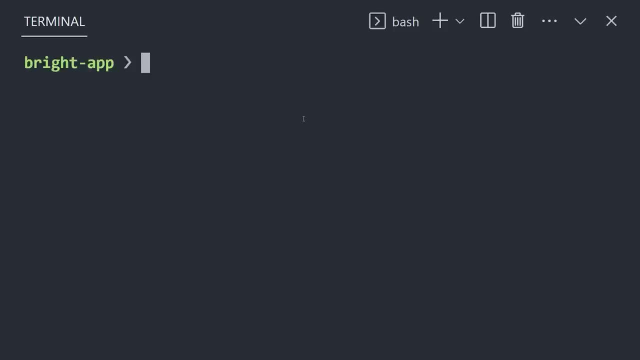 using it, Then your mom will be pissed that she can no longer order her groceries from Walmartcom. That's where the scraping browser comes in. It's a remote browser that uses the proxy network to avoid these problems. To get started, I'm creating a brand new Nodejs project with NPM. 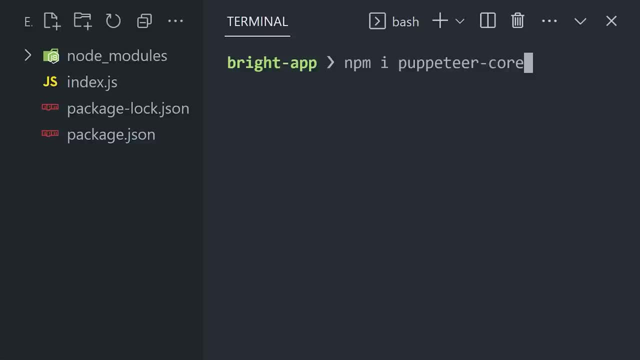 then installing Puppeteer- Well, actually Puppeteer Core, which is the automation library- without the browser itself, because again, we're connecting to a remote browser. Go ahead and create an indexjs file and import Puppeteer From there. we'll create an async. 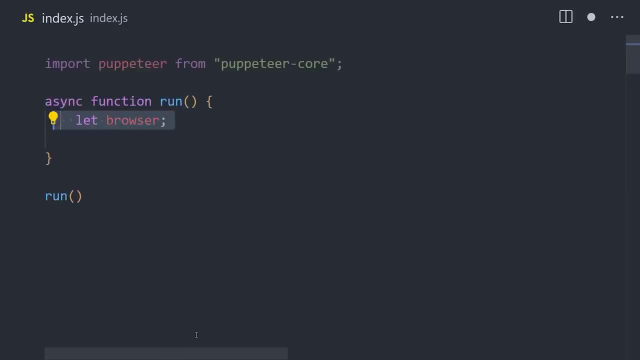 function called run that declares a variable for the browser itself. Inside this try-catch block, we'll try to connect to the browser. If it throws an error, we'll make sure to console log that error And then, finally, when all of our scraping is done, we'll want to automatically close the. 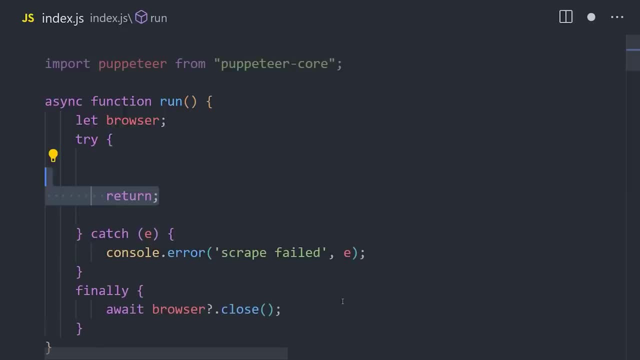 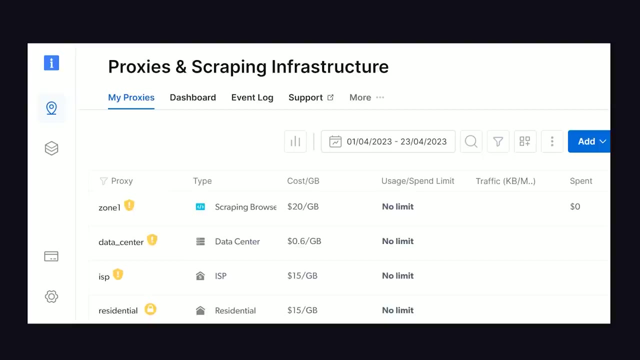 browser. You don't want to leave the browser opened unintentionally. Now, inside of try, we're going to await a Puppeteer connection that uses a browser WebSocket endpoint. At this point we can go to the proxy section on the BrightData dashboard. 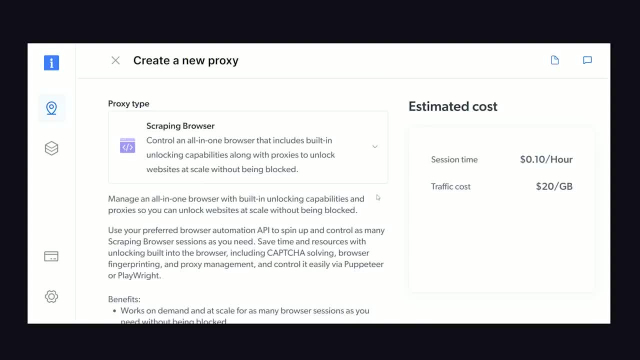 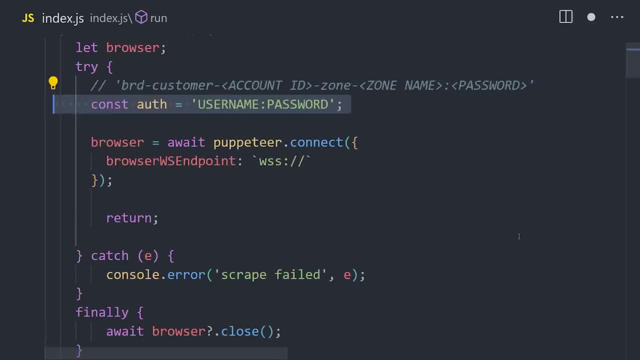 create a new scraping browser instance. Once created, go to the access parameters and you'll notice a host username and password. Back in the code we can use these values to create a WebSocket URL. You'll have your username and password separated by a colon, followed by the 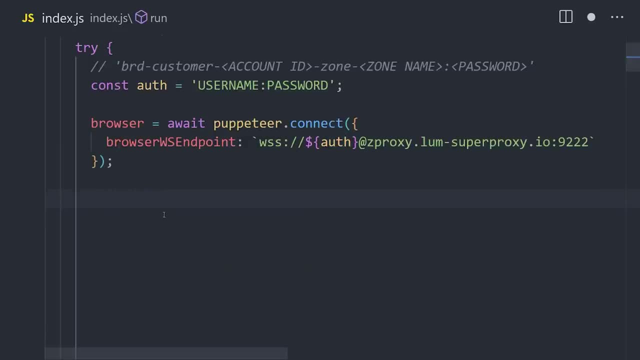 host URL. Now that we're connected to this browser, we can use Puppeteer to do virtually anything a human can do programmatically. Let's create a new page and then set the default navigation timeout to two minutes. From there, we can go to any URL on the internet. Then Puppeteer has a variety of 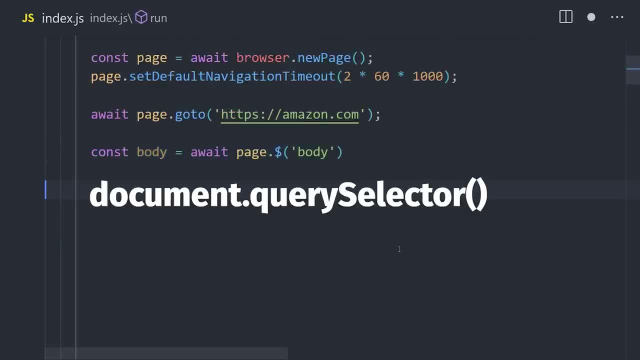 ways to create a page like the dollar sign, which feels like. jQuery corresponds to document query selector in the browser. It allows you to grab any element in the DOM then extract text content from it, Or, as an alternative, you can use page evaluate, which takes a callback function. 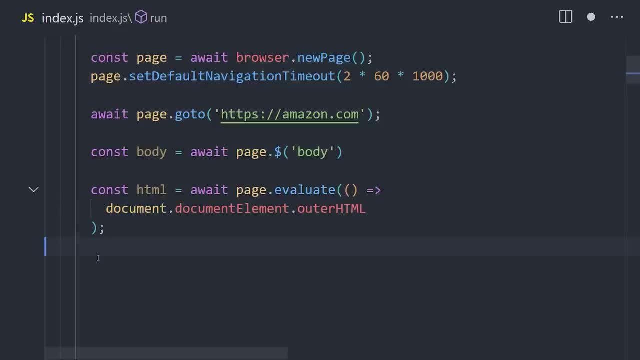 that gives you access to the browser APIs directly, Like here. we can grab the document element and get its outer HTML, just like you might do in the browser console. Let's go ahead and console log the document's outer HTML, And now we're ready to test our scraper out to make sure everything's. working as expected. Open up the terminal and run the node command on your browser. Now we're going to test our scraper out to make sure everything's working as expected. Open up the terminal and run the node command on your browser. Let's go ahead and console log the document's outer HTML, And now we're ready to test our. 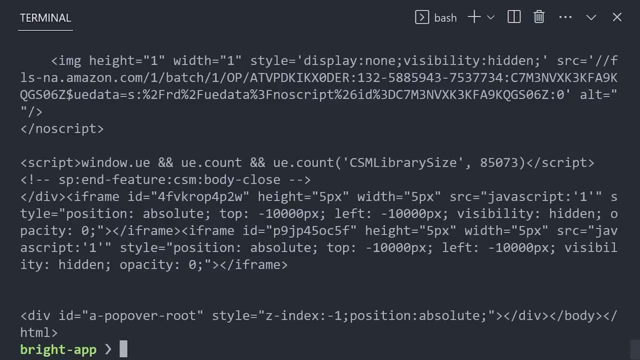 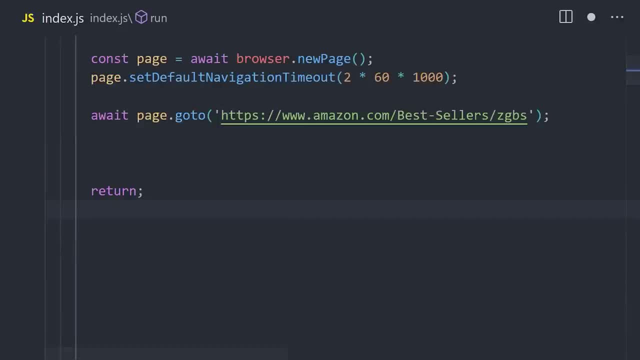 file, And you should get the HTML for that page back as a result. Congratulations, you're now ready to do industrial scale web scraping. Now I'm going to go ahead and update the code to go to the Amazon bestsellers page, And my first goal is to get a manageable chunk of HTML. What I'm doing is opening: 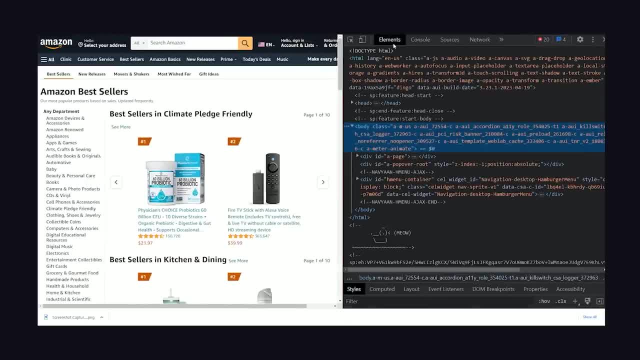 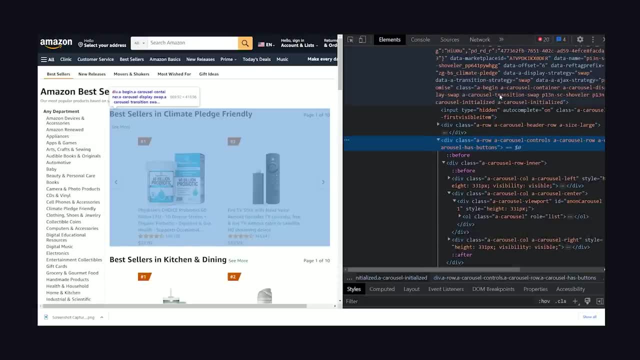 up the browser dev tools in Chrome to inspect the HTML directly until we highlight the list of products that we want to scrape. Ideally, we'd like to get all these products and their prices as a JSON object. You'll notice all the products are wrapped in a div that has a class of a. 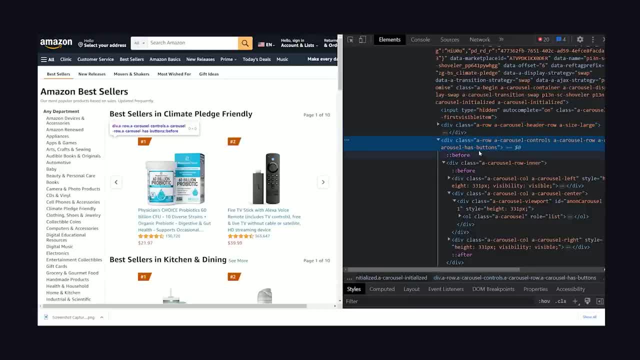 carousel. We can use that selector as our starting point And we can also use it to copy and paste the HTML into the chat. Chrome dev tools also has a copy selector feature, which is pretty cool, but usually it's a bit of overkill Back in the code. we can make sure that. 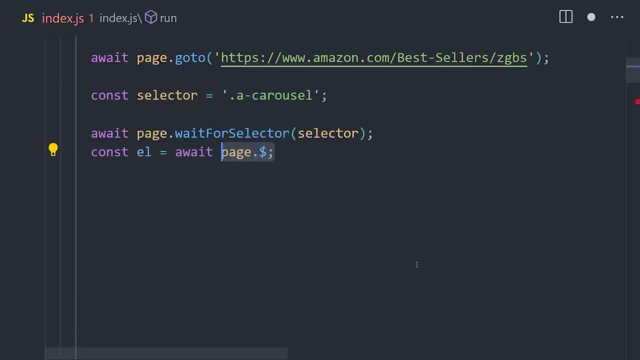 the page will wait for that selector to appear. Then we can use the dollar sign query selector to grab it from the DOM and finally evaluate it to get its inner HTML. Now let's go ahead and console log that and run the script once again. At this point we have a more manageable chunk. 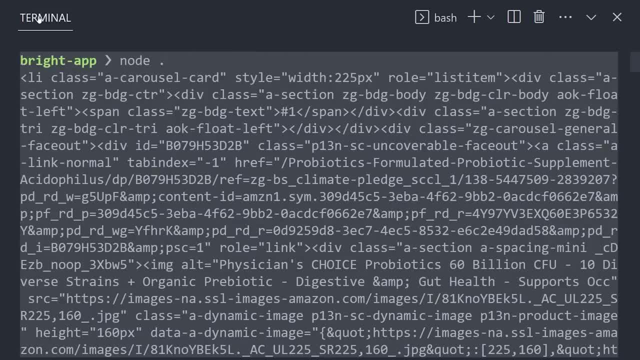 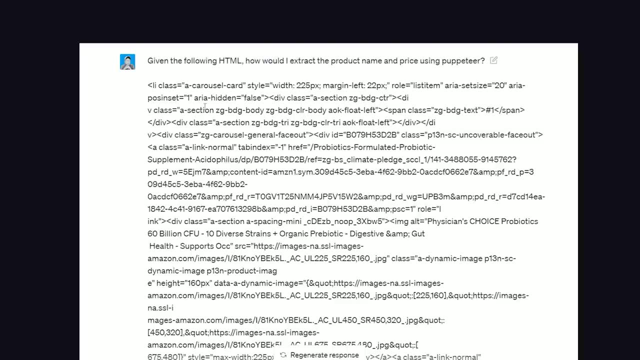 of HTML and I could analyze it myself, But the faster way to get this job done is to use a tool like chat GPT. We can simply copy and paste this HTML into the chat and ask it to write puppeteer code. that will grab the product title and price and return it as a JSON object. Literally on the 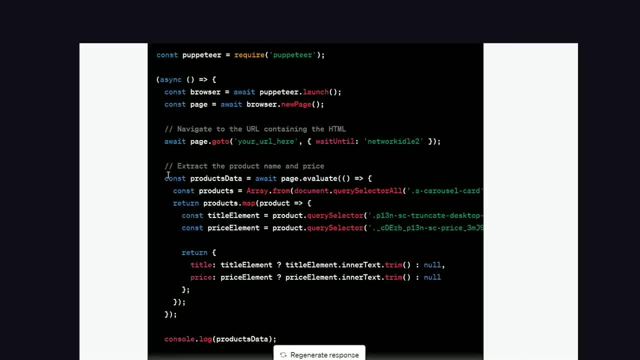 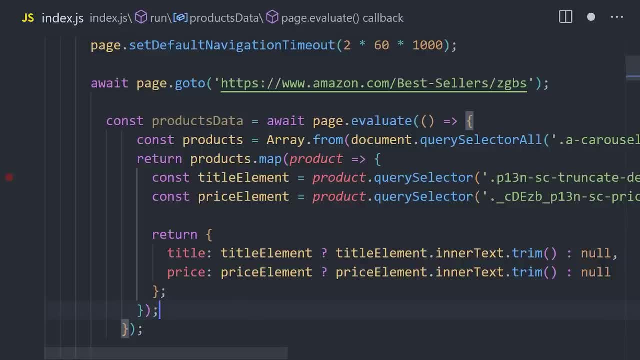 first try. it writes some perfect evaluation code that grabs the elements with the proper query selectors and then formats the data we requested as a JSON object. Let's copy and paste that code into the project and then run the node script once again. Now we're in business. We just